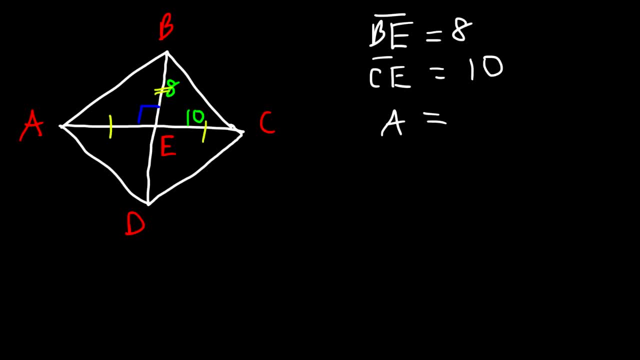 are perpendicular to each other. So AE and EC are congruent and BE is congruent to ED. So therefore that means that ED is 8 and AE is 10.. So now we have the length of the two diagonals. So diagonal AC is 10 plus 10 or 20 units long and diagonal BD is 8 plus 8 or 16 units long. So we 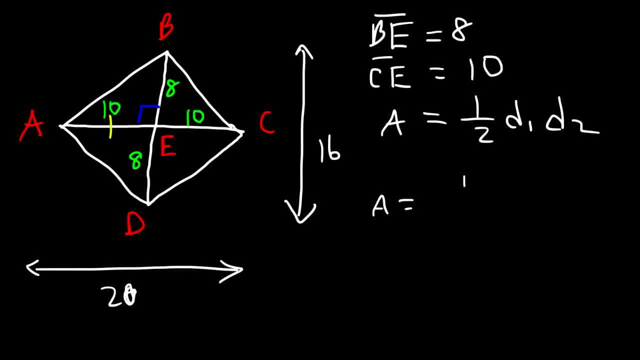 could use this formula again: It's 1 half D1 times D2. So D1 is 16 and D2 is 20.. Half of 16 is 8 and 8 times 20. If you have eight $20 bills, you have 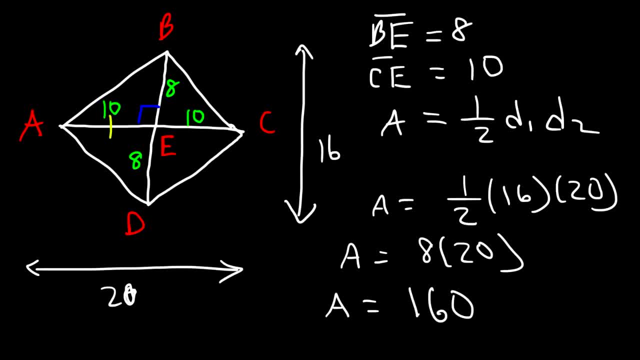 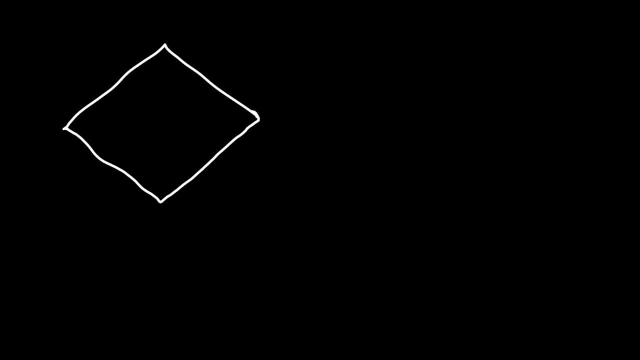 160 bucks. So this is going to be 160.. And so that's another way in which you can calculate the area of a rhombus. if you're given those two sides, Here's another problem for you. So, given the same type of rhombus, rhombus A, B, C, D. 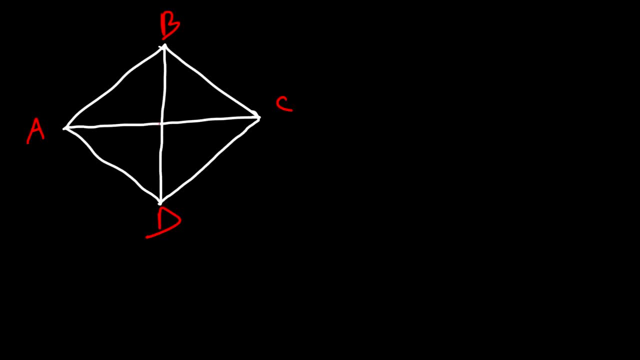 I'm once again going to say: this is point E. Let's say, if we're told that CD is 17 units long and AE is equal to 8. Calculate the area of the rhombus. So AE is 8. And CD is 17.. How can we calculate the area with this given information? 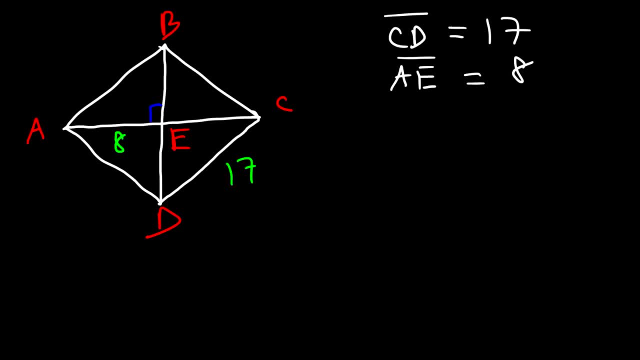 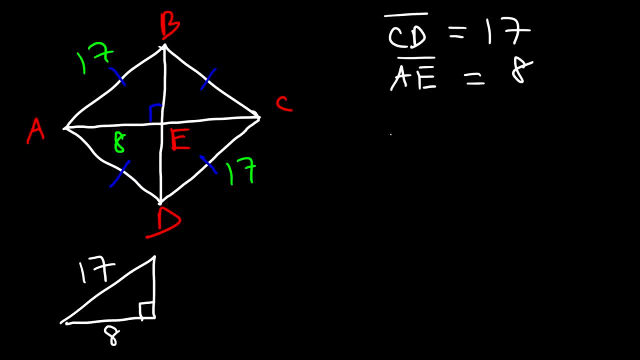 The hypotenuse is 17 units long and AE is 17 units long And the base is 8.. What is the height? How can we figure this out? So we need to use the Pythagorean theorem C. the hypotenuse is 17.. 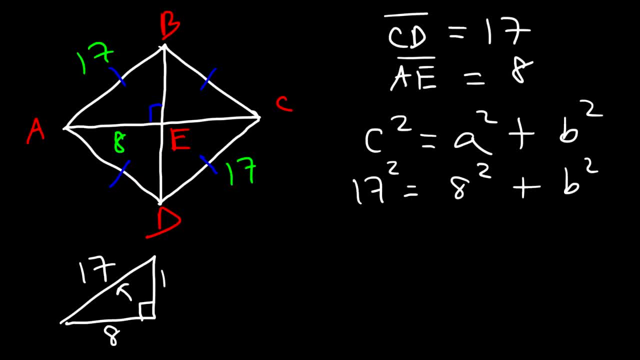 A is 8.. Now let's calculate B: 17 squared, That's 289.. 8 times 8 is 64. Now 289 minus 64 is 225.. And so that's equal to B squared, And if we take the square root of both sides, the square root of 225 is 15.. 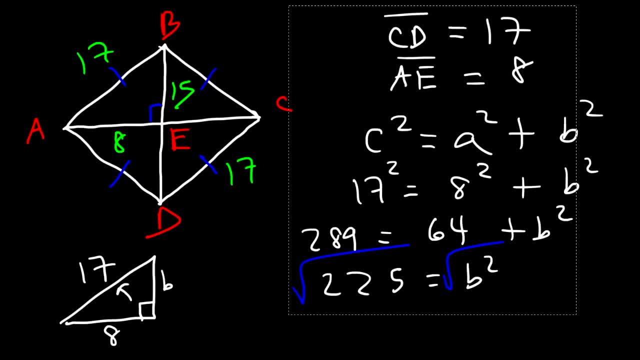 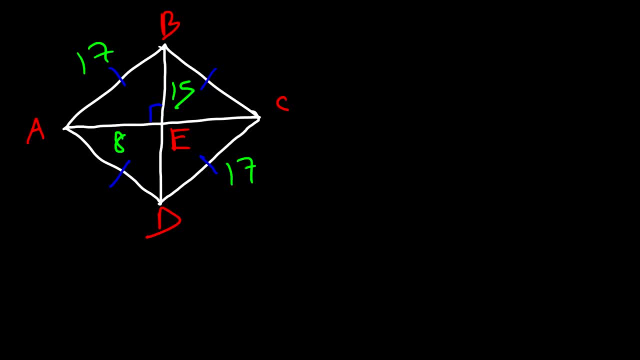 So BE is 15 units long. So now we can calculate the area. So if BE is 15. That means ED is 15. And if AE is 8, EC is also 8. So this diagonal is going to be 8 plus 8, or 16 units long. 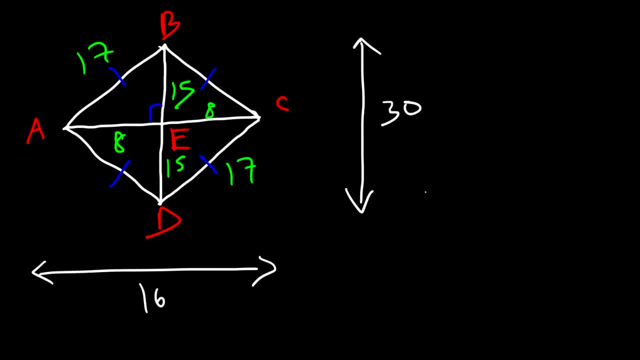 And this one is 15 plus 15, or 30 units long. So the area is 1 half D1 times D2. So that's going to be 1 half times 30 times 16. So half of 30 is 15.. 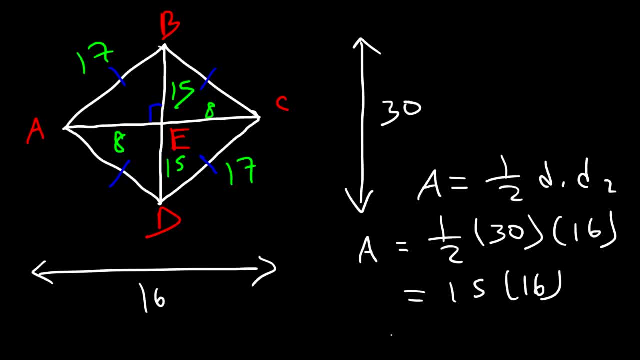 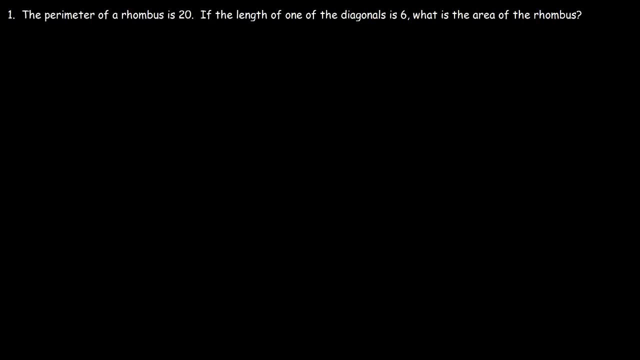 15 times 16.. That's 240.. And so that's the area of this particular rhombus. It's 240 square units. The perimeter of a rhombus is 20.. If the length of one of the diagonals is 6,, what is the area of the rhombus? 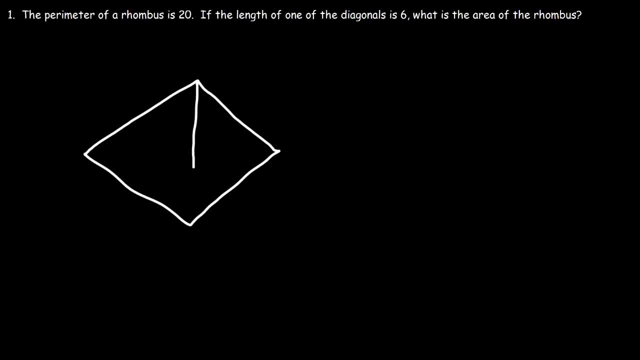 So let's draw a picture. So if we're given a perimeter, what is the side length of the rhombus? Keep in mind that all four sides are congruent. So if this is S, then all sides are S, So the perimeter is simply 4S. 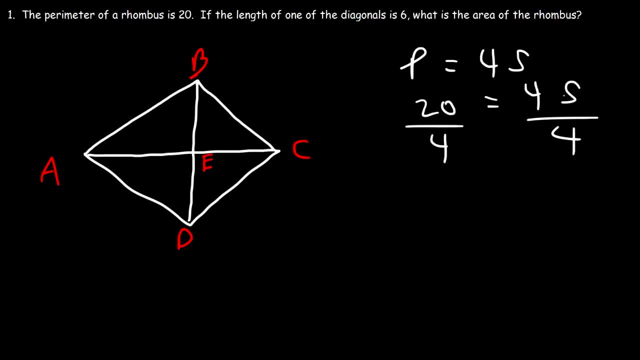 So all we need to do is divide the perimeter by 4, and that will give us the side length of the rhombus. 20 divided by 4 is 5.. Okay, So this is 5 units long. Now the length of one of the diagonals is 6.. 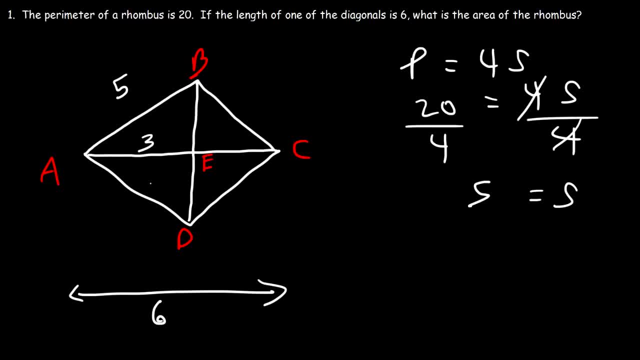 So let's say AC is 6.. That means that AE is 3.. And EC is also 3.. So now we can calculate the missing side of the right triangle. We can calculate BE. So C squared is equal to A squared plus B squared. 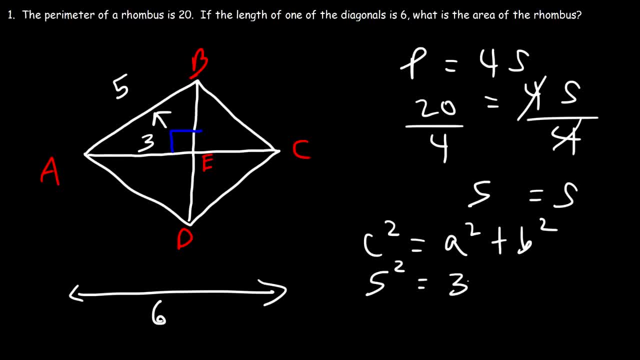 C, the hypotenuse is 5.. A is 3.. So let's calculate: B: 5 squared is 25.. 3 times 3 is 9. And 25 minus 9 is 16.. So 16 is equal to B squared. 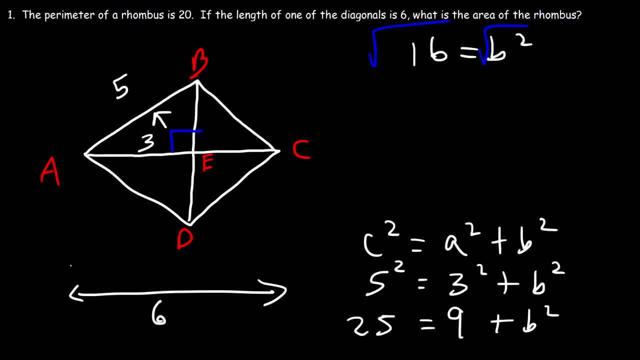 And now let's take the square root of both sides. So the square root of 16 is 4.. So we have a 3,, 4,, 5 right triangle. So now we can calculate the area. So if BE is 4,, ED is 4.. 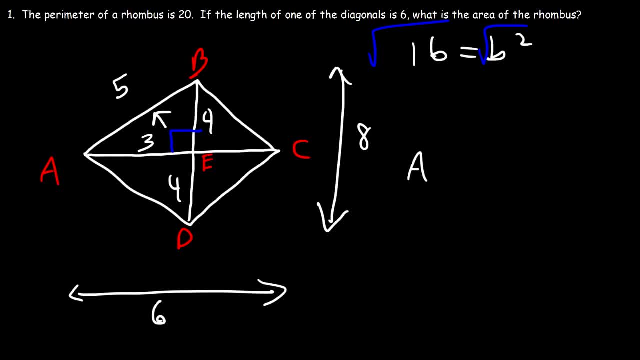 Which means that diagonal BE is 4.. And the diagonal BD is 8.. So the area is going to be 1 half D1 times D2. So that's going to be a half times 8 times 6.. Now half of 8 is 4.. 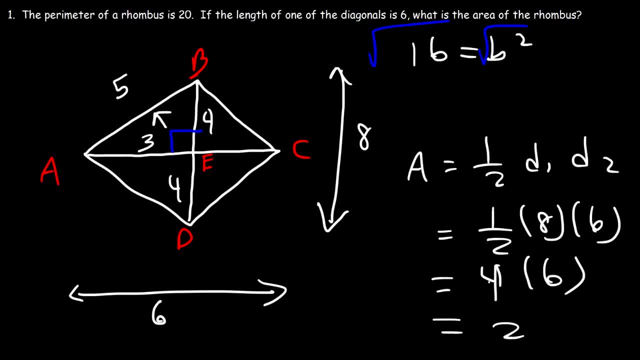 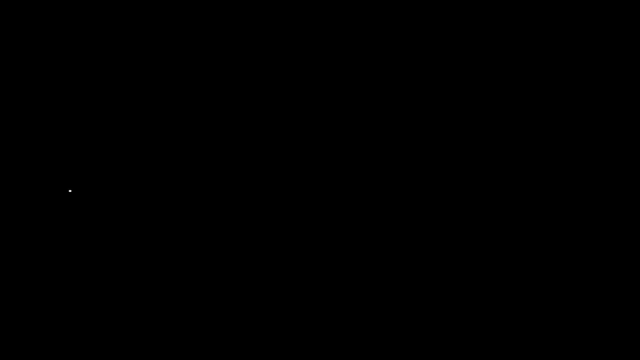 And 4 times 6, that's 24.. And so that's the area of this particular rhombus. It's 24 square units. Now let's see, Okay, Now let's say this side is 30. And let's say this part is 15.. 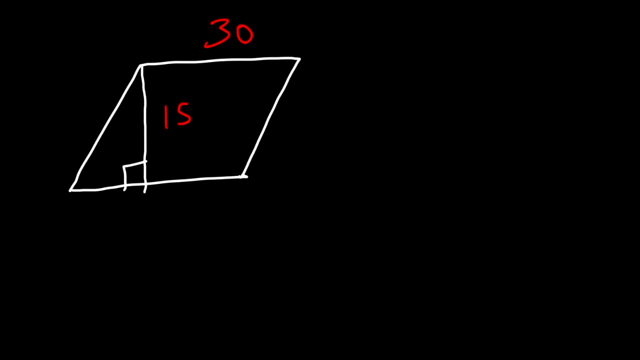 What's the area of this rhombus? So what do you think we need to do Now? you need to know that a rhombus is a type of parallelogram, And so a square is a parallelogram as well. A rectangle is a parallelogram. 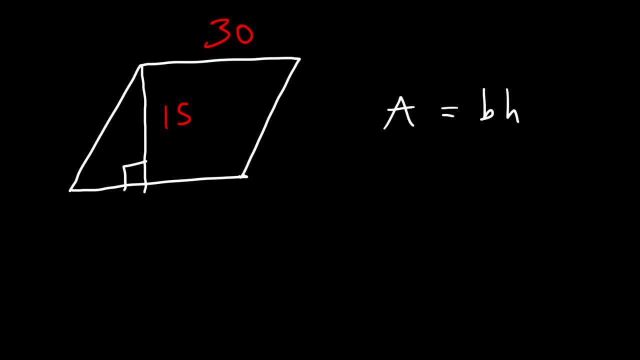 And the area of any type of parallelogram is the base times the height. In the case of a rectangle, the area is length times the width, But you can also treat this as base times height. You get the same thing. For a square, the area is S squared or S times F, which is also base times height. 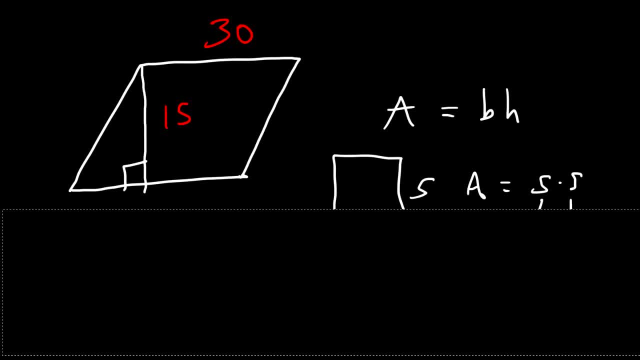 So for any parallelogram, whether it be a rectangle, a square or rhombus, you can also use a rectangle, a square or rhombus. The area is base times height. So the base of this particular rhombus or parallelogram is 30.. 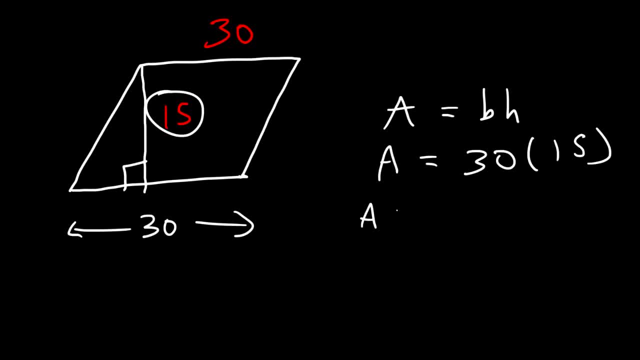 And we can see that the height is 15. So the area is just 30 times 15. And so it's 450 square units. Try this problem. Okay, So let's say, if we have rhombus A, B, C, D, And let's say that B, C is, let me think. 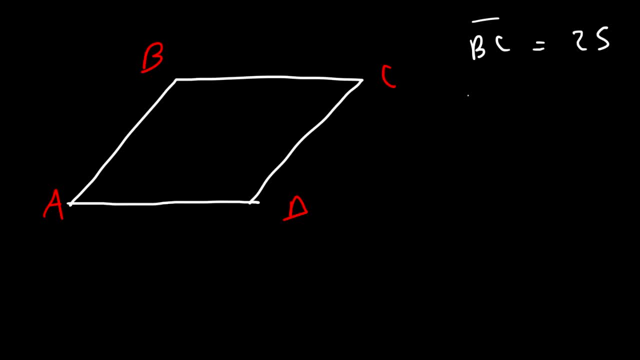 about this. Let's say B C is 25 and B D is 24.. Actually, let's make B D 14.. So if B C is 25 and B D is 14. Okay, That is 65 and B is 25.. 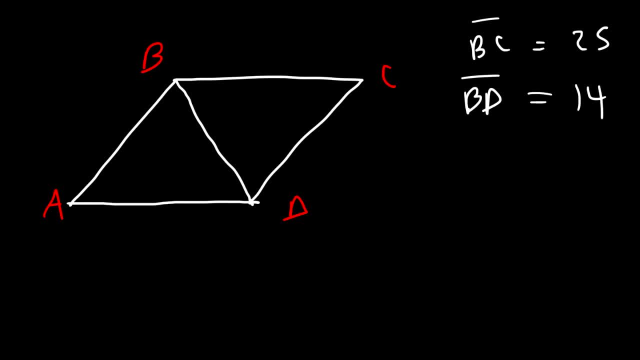 Let's add two more numbers, So 27, and B is 14.. We need a: 3.. All right, Next up we have the square. Actually, let me twice check what I didn't write. Okay, 1,0.. 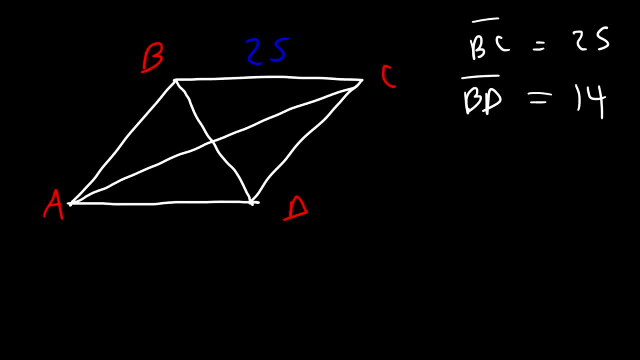 1,0,1.. Let's see 1,0.2.. L robs 16.1.. hologram Now: if BC is 25 and if BD is 14, that means BE has to be 7 and ED has to be. 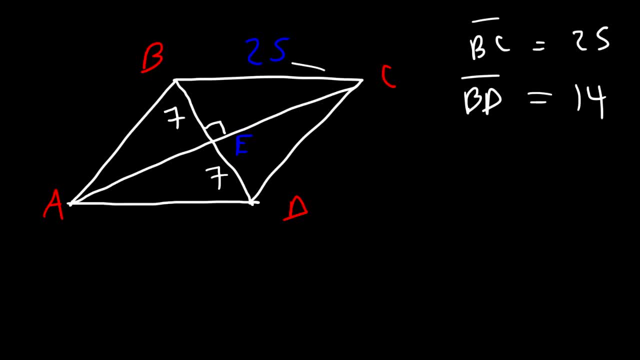 7 as well. So now we just got to find the missing side of this right triangle. So the hypotenuse is 25.. The height of that triangle is 7.. Let's calculate the base of the triangle. So C squared is A squared plus B squared, C squared is 25.. A is 7. And B is. well, we're.